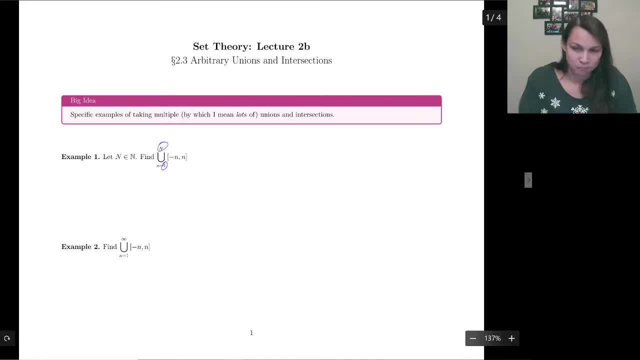 For everything, one up to some arbitrary capital N, where capital N is coming from the natural numbers. So we're talking about: first we would have this interval, Next we would have this interval, And then we would have this interval all the way up to some interval that we don't know. 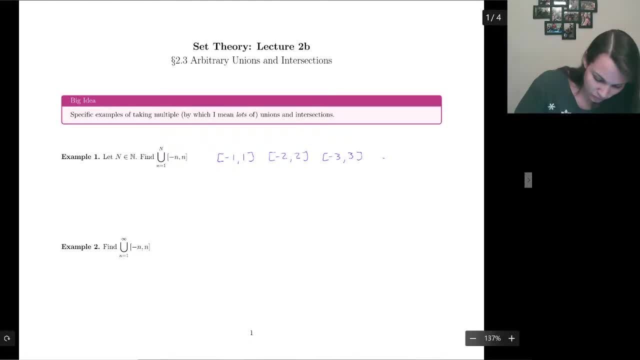 Some capital N. So the key right here is to notice that our intervals are getting bigger. So this first one is contained in the second one, And the second one is contained in the third one And that is contained all the way here in the very last one. 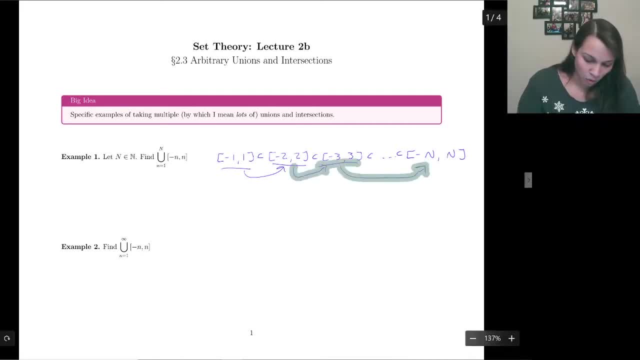 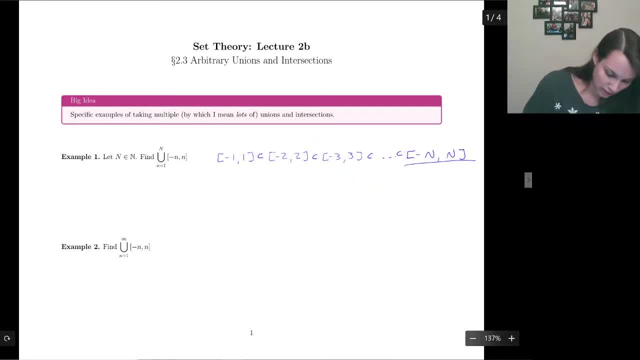 All of them, All of these guys previous. So our union here is just going to be Negative N, The positive N, Or we're using the capital N. And the reason that it's good to like kind of think about that first is what, if we wanted to look at, 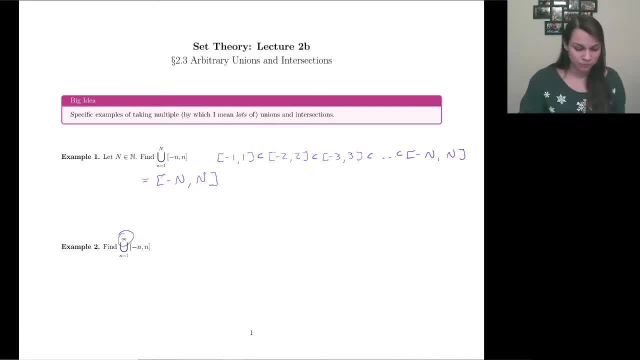 Infinitely many unions. So we're going to go all the way up to infinity. Well, we know that The Limit Of N Would just be infinity, As N goes to infinity, And the limit of negative N, As N goes to infinity. 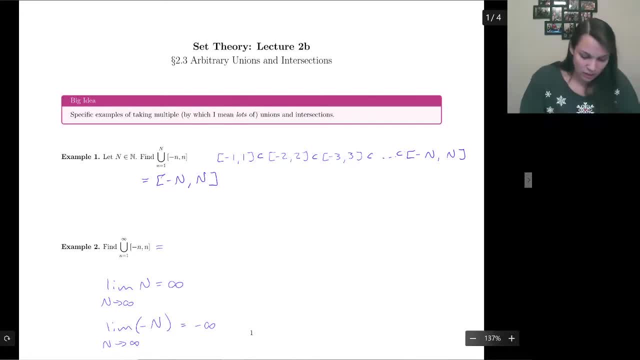 Would be negative infinity And then we just plug in that limit for our endpoints. So we would go to negative infinity, Positive infinity And hopefully me writing that makes you go. Ah, Don't do that. Remember we can't equal infinity. 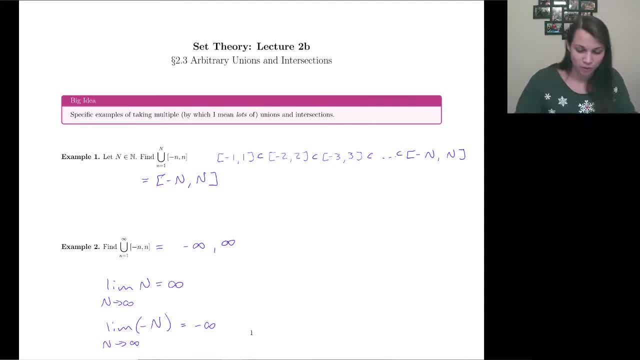 We don't want to include infinity. That's like a topic for a much different, Much higher course. Including infinity, Actually equaling infinity. That's not what we do here- Cannot equal infinity, And so, remember, you're always going to use those round brackets for infinity. 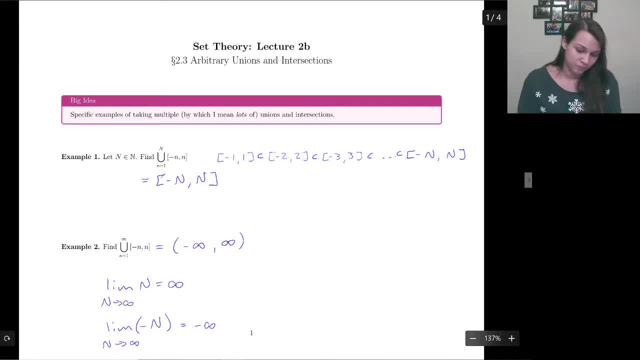 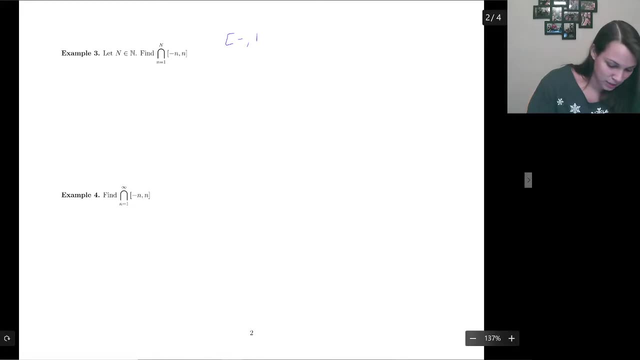 Even if we did start with square brackets. Okay, So that's Basic union. Let's go ahead And do A Intersection Once again. I'm going to write this down Up here Just to help myself visualize. And so we're going to do intersection. 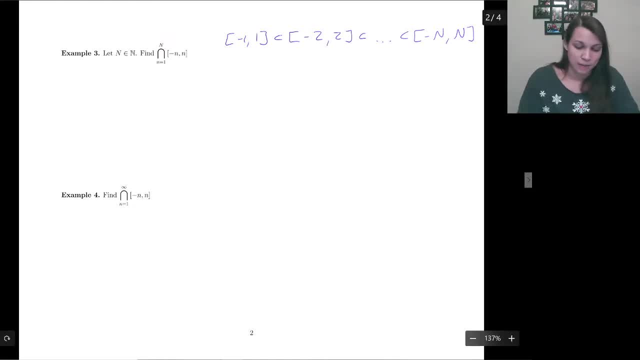 Same interval And we're going to go up to capital N, So the intersection is everything that everybody has in common. So this one Is the smallest and he's contained in all of these ones, And so we can take our smallest interval because he's contained in all the other ones. 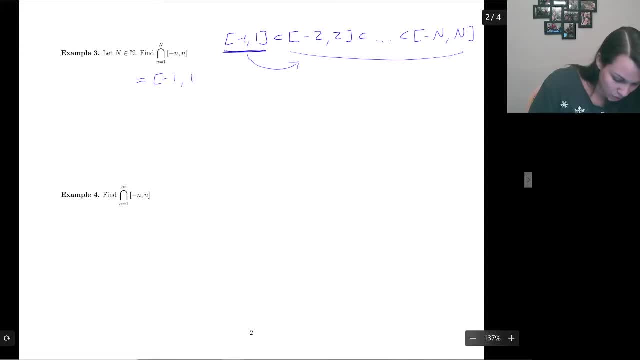 And say, okay, Negative one to one Is what everybody is going to have in common. So now, when we take an infinite Intersection, We don't care. We don't care where this Big one goes, We only care about the smallest. 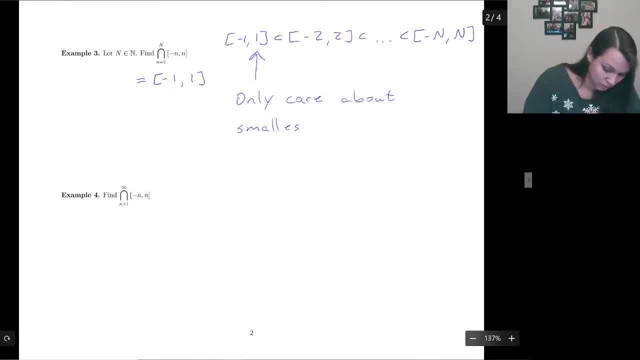 We only care about smallest For the intersections. So this guy can get as big as he wants. He could go all the way up to all of infinity, to negative infinity, But we only care about what everyone has in common, which is that smallest one. 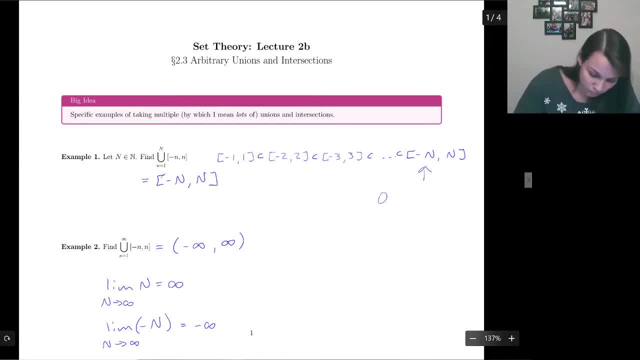 And then We can leave a similar Out here, Only Care About largest For the union. And again, this is only because they're nested, They're contained inside of each other. Okay, So let's take this on a run again. 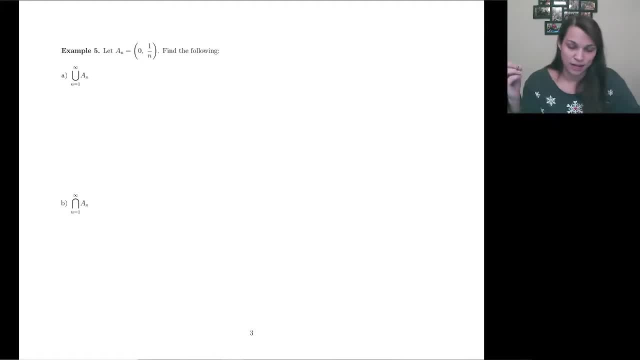 Let's try A different set of, And we're going to do the interval zero to one over. And I am going to start again By writing out some intervals. So if n was equal to one, Then we would have. And is equal to two. 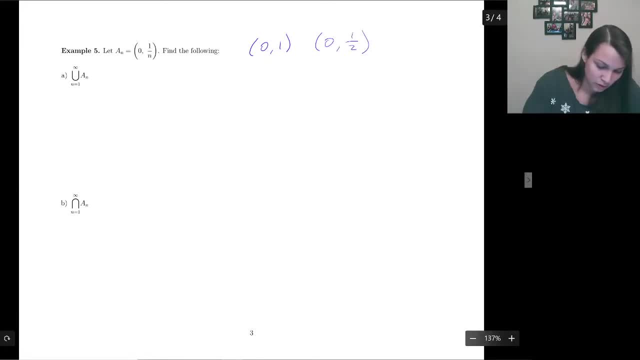 Like: this is a one, This is a two. Let's write out a three: Zero to one third. Now we have set containment Going the other way. Now this one is the largest, And this one is the largest, And this one is the largest. 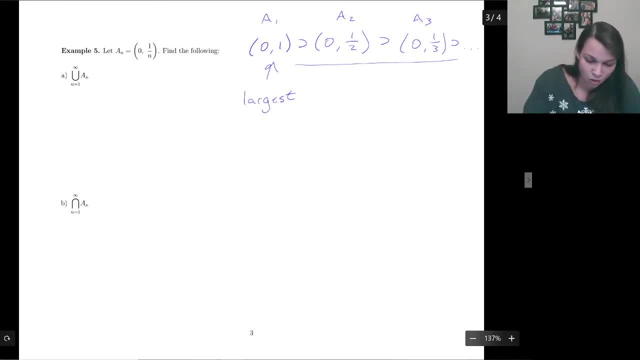 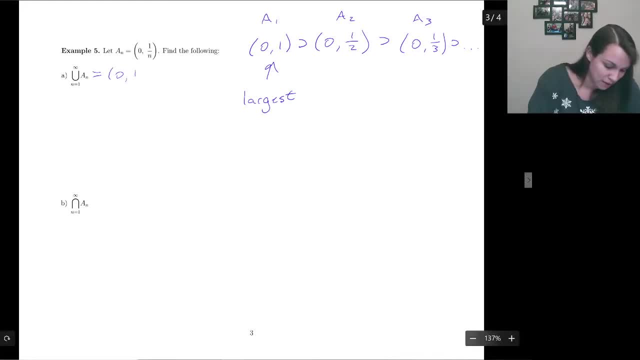 And so our union Is going to be everything between everybody, Which is just going to be the biggest one. Now remember, for intersections, We care about the smallest, So the question is, What is the smallest one Doing? So we're going to take a limit. 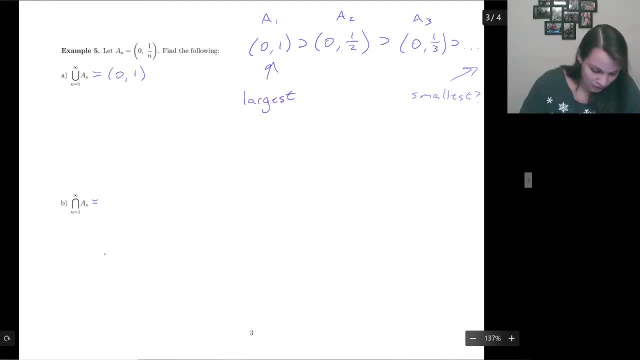 And say: well, let's figure out Essentially If I get that big N back, So the smallest one Would be This interval right here, And I need to know What this is doing As big N Goes to infinity. So what does? 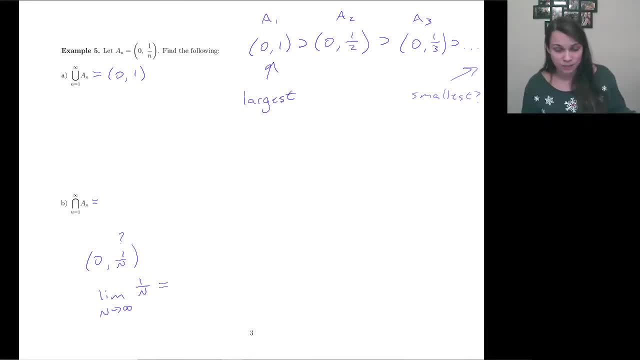 One over big N, As N goes to infinity, do It goes to zero. So then we're left with Going to write something really bad. We're left with the interval Zero to zero. No, That's not an interval, That's just. 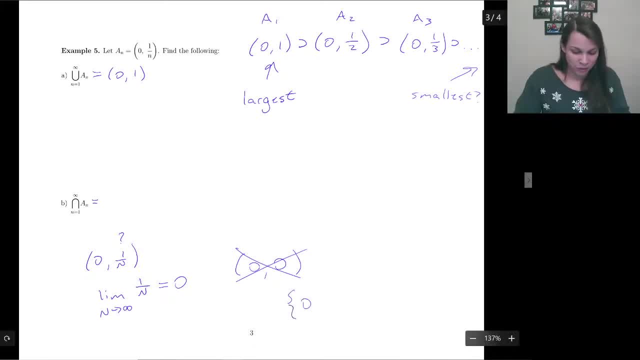 The question is: Is it just a single point? Is it just the point zero? No, Because round means We don't include, So we're not including zero, Which means we could. This endpoint Can't get small enough to go pick up that zero. 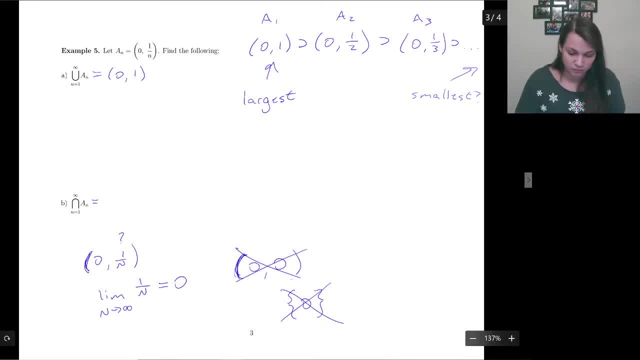 We already said on this side, We're not going to include zero, So that means We have the empty set. There's nothing in here. If I'd had square brackets, So this interval instead, Then we would have Taken a limit and gotten. 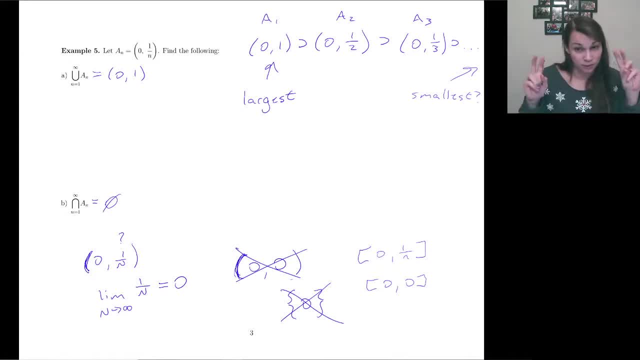 This, So we would be including zero On both ends of our Interval, And so that would be. That would turn into this. So if I had square brackets And I had included zero, I would have ended up with Just the element zero. 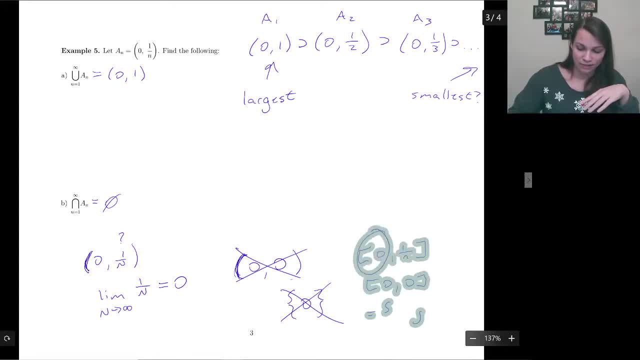 In our intersection. But that is not the case. That is not what has happened. Okay, So What we had was the Interval zero to zero, with Round brackets, Which means we have nothing sitting in there. So this is bad notation. 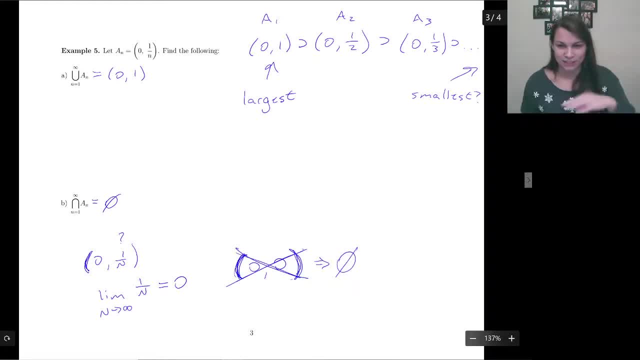 We don't write this, We write empty set. That is the conclusion. Okay, Now let's try Another one Where we have some very Interesting notation. We have A is an interval. again, It is cool, But now we have this set. 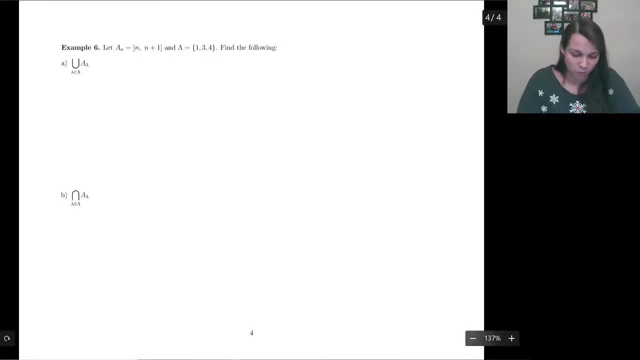 Lambda, Which is equal to one, three and four, And we are going to union Over The lambdas From The capital lambda. So the reason I am doing this Is because it is notation that you guys need to know. It is like hard to like. 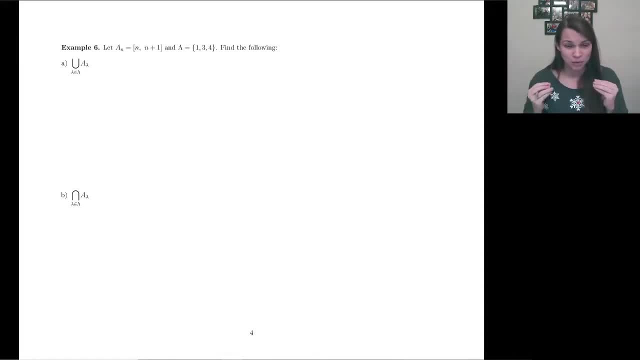 Think about, And so we are just going to stay really simple Right now, In hopes that I can prepare you for your futures, Where you have to look at this And make sense out of it. So let's dig into this. 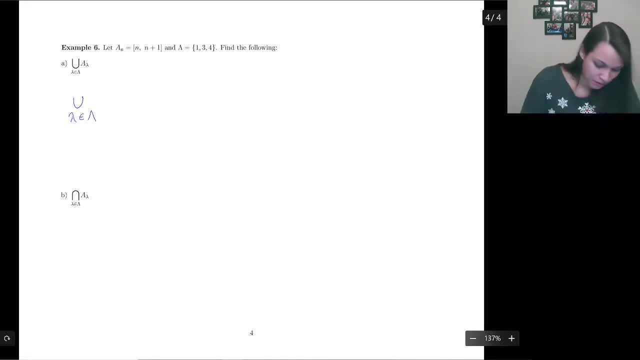 What is this trying to say? So this union of lambda in Capital, lambda Just means that Lambda is going to be equal to one, Three Or four. So our union Is going to be between A one Union, A three. 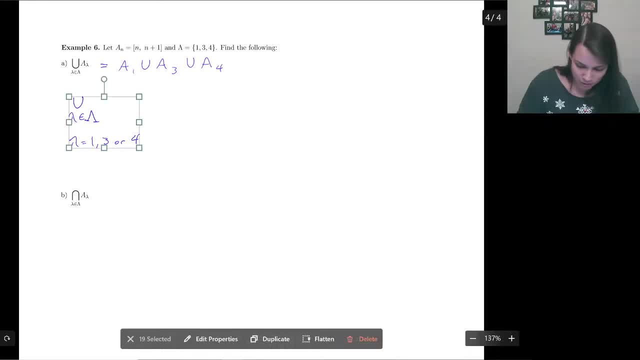 Union A four. It is a very complicated way to say that, But trust me, Being able to do that arbitrary Notation Is really important later on. So then the questions are: Well, what is A one, A three? 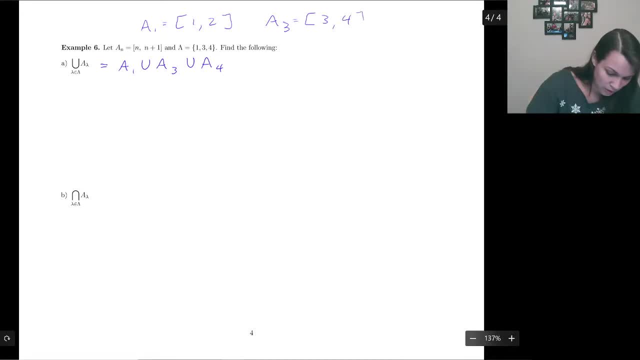 And a four. Three to four. A four is the interval Four To Five. So then The union Is going to be This interval Glued together with this interval, Glued together with this interval. I am not looking for what is the biggest. 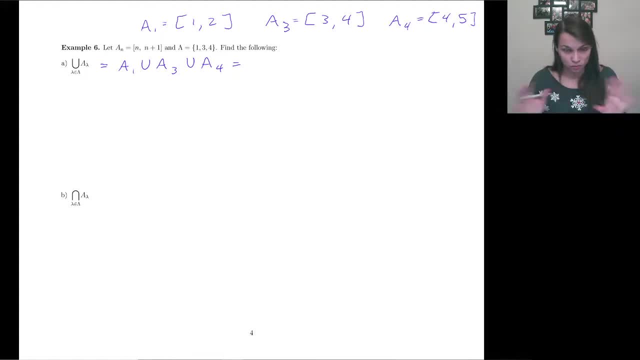 What is the smallest? Because these are not nested intervals Anymore, Glued them together like we normally would. So that would be One, Two, Union Three, Four, Union Four, Five. And if Let's say this was an exam, 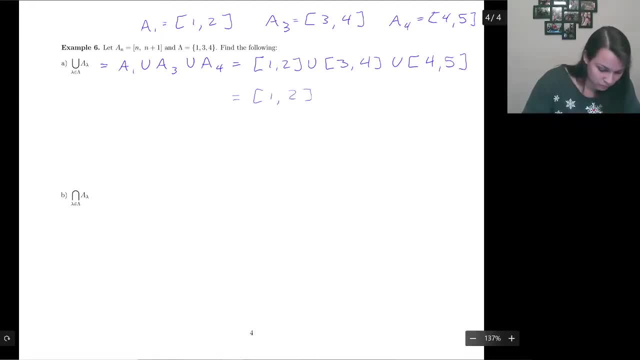 And this is where you stopped. You would get some of the credit. There we go. We cannot pretty up this Notation. There is nothing. There is no way to like More concisely, write this: So we are done for the union. 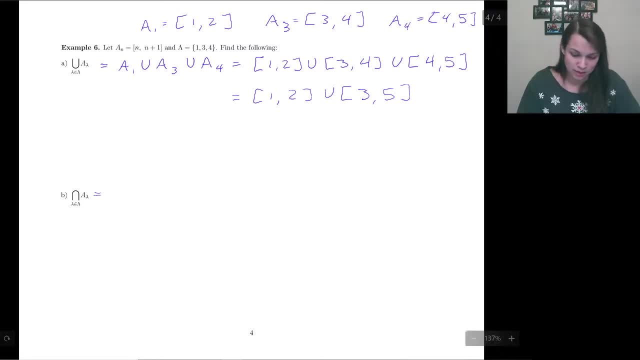 Okay, so intersection. Let's say we are going to do The intersection Between a one, A three And a four. So this Is when we want to know What these intervals Have in common. So we look Here: 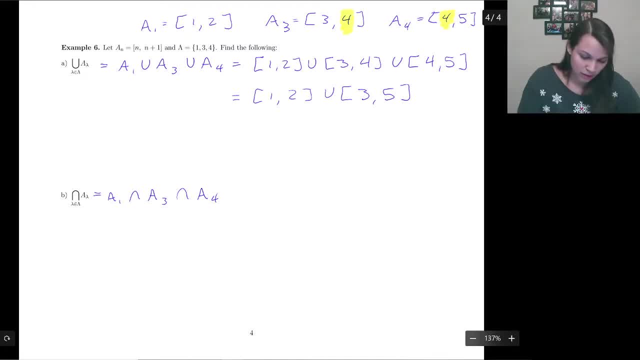 We look here And we can say, Oh, They have this Four element in common. And then we look here at a one And say There is no four, So They don't have any elements in common at all. Their intersection: 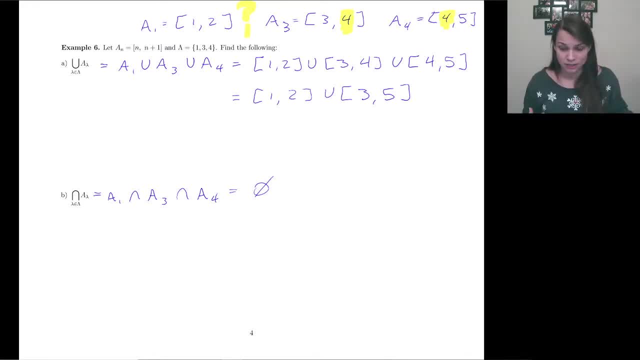 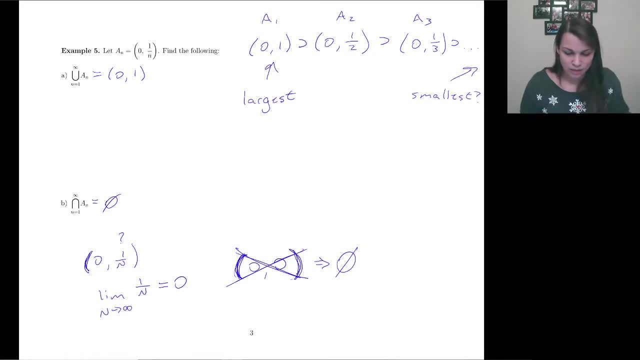 Is just Some new notation. It was dealing with some- Oh my goodness, Slide back, There we go. It is dealing with some Infinitely many unions And intersections. Yes, I need some explanation with this, But this is all the explanation. 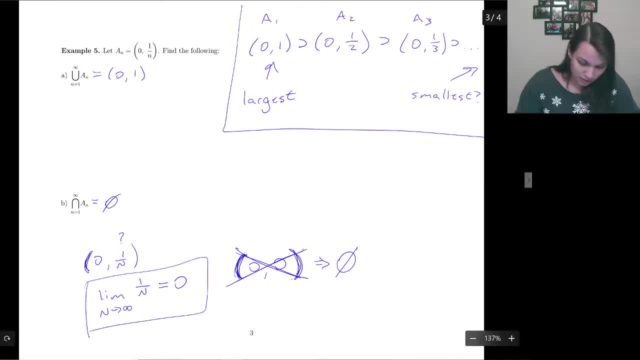 That I really need Between there And there, Like, if you can show me, You can see That the Intersections Are large over here And they are getting smaller As we go this way And then you take a limit.